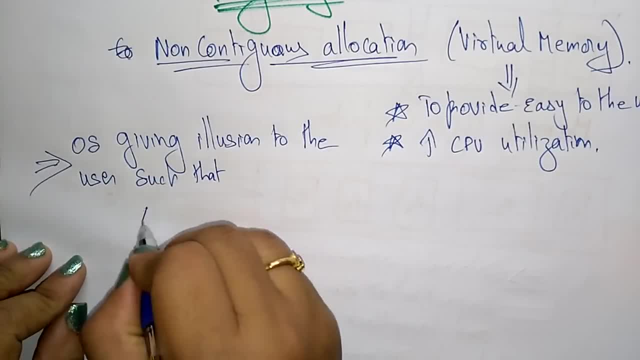 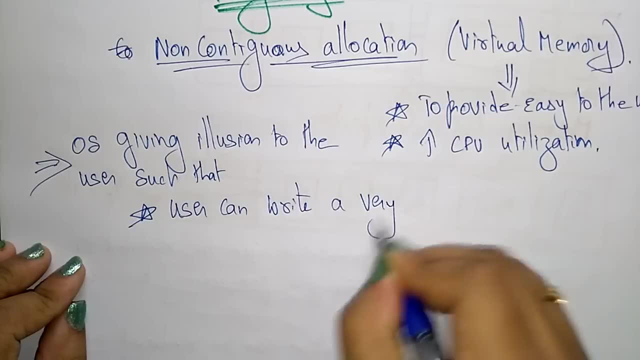 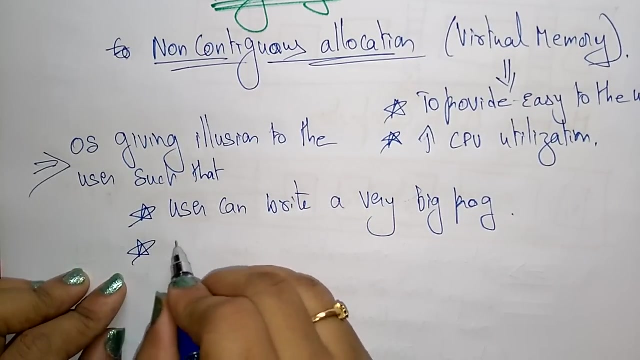 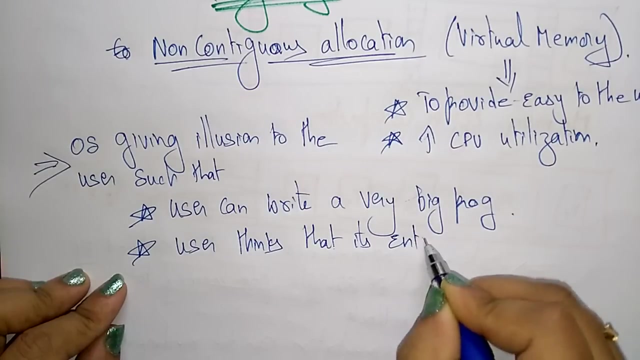 So let me write a that it's entire program program is present in RAM. So just the user. the user can write a very big program and user thinks that it's entire program program is present in RAM. So just the user think that the entire program, whatever the program that he is axing that is present in ram. 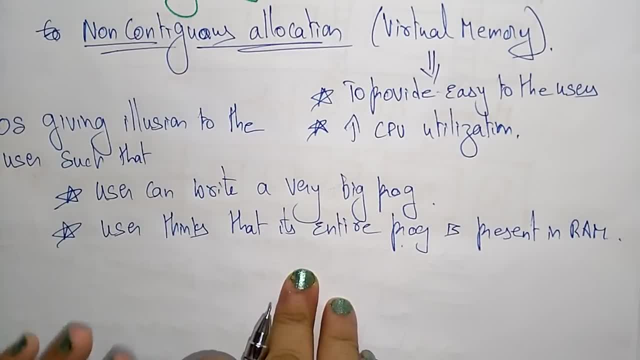 so he is just the watch. i'm saying about the virtual concept, virtual memory, which is a non contiguous allocation. so here the operating system is giving just illusion to the users. why it is? giving uh, illusion to the users means we are using the virtual memory to user can create a very big 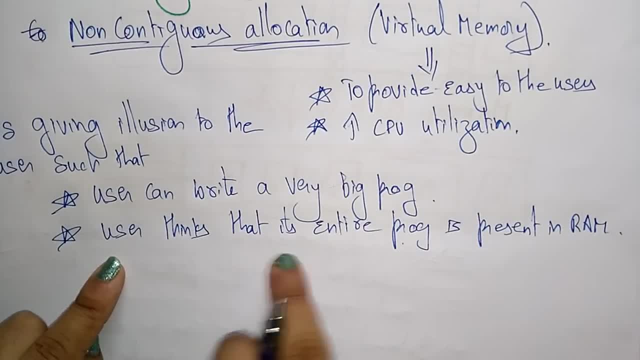 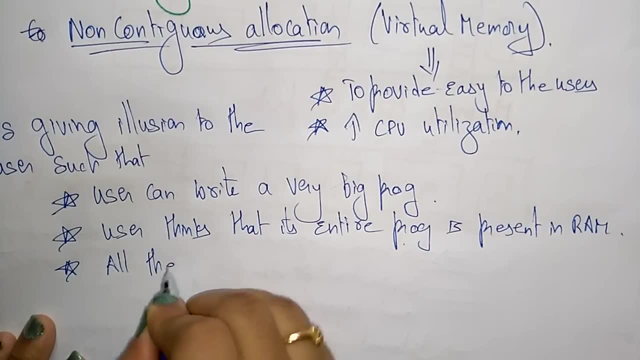 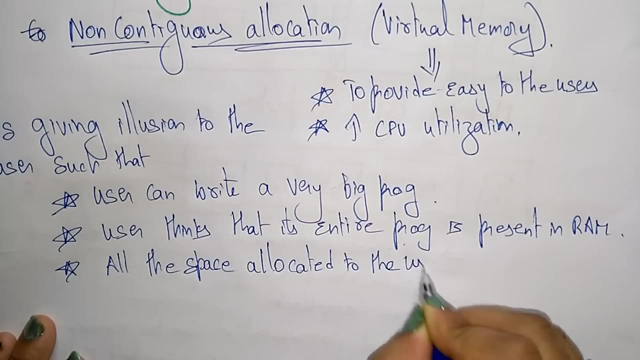 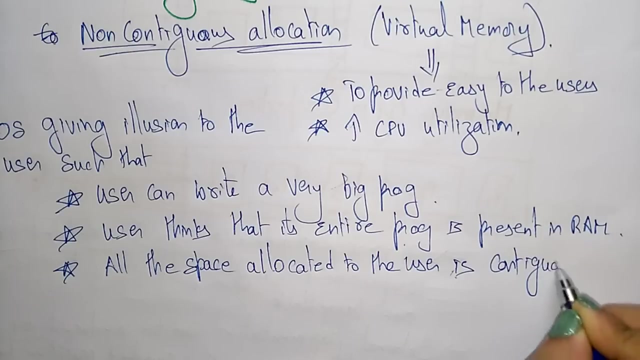 program with the help of virtual memories and also user thinks that its entire program, whatever he is axing, is present in ram and all space, all the space allocated to the user is contiguous. so it is thought that that whatever the space that is allocated in the main memory is contiguous and user address starts from all zeros. so it's just creating illusion to 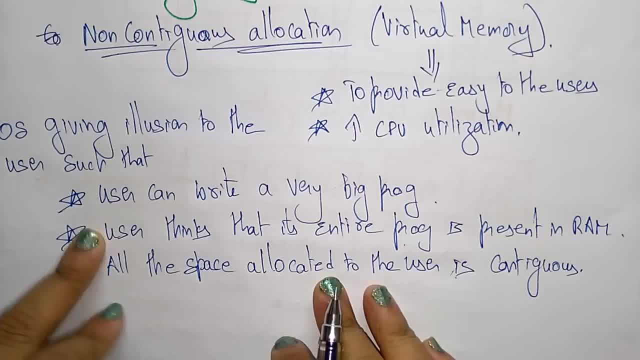 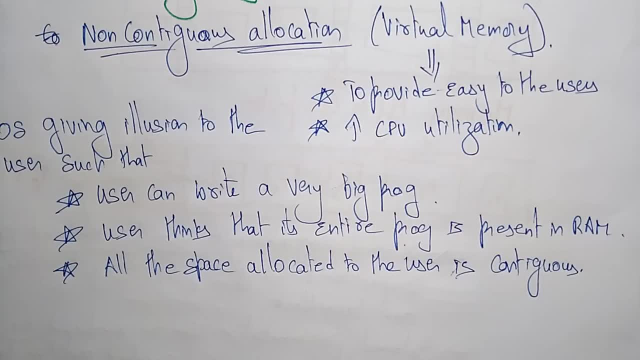 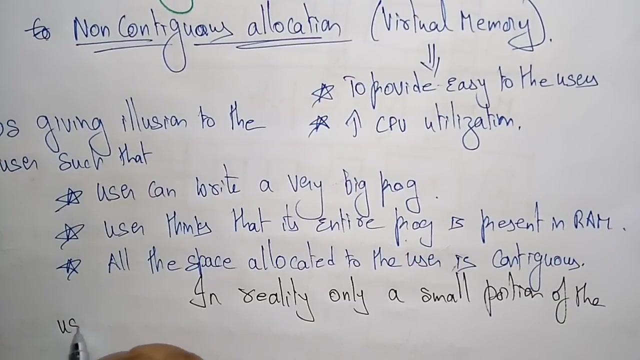 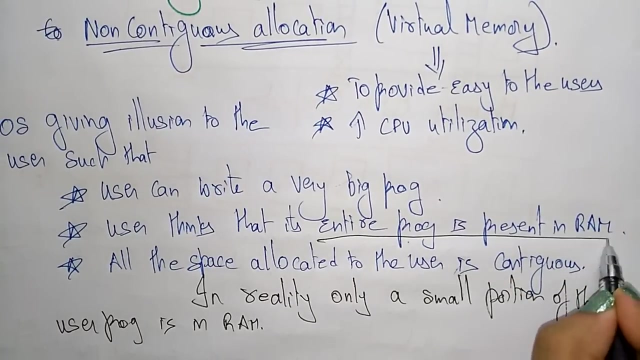 users by using this poignant to alert that user can write a very big programs and users can think to and write entire program in ram. so in reality, actually, in reality, in reality, only a small portion, only the small portion of the user program is in ram. so in the ram not the entire program is present in the ram. 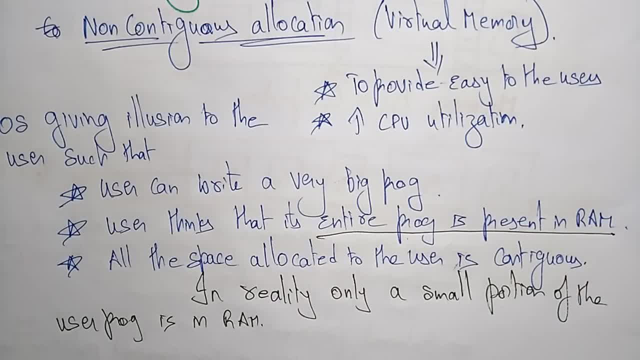 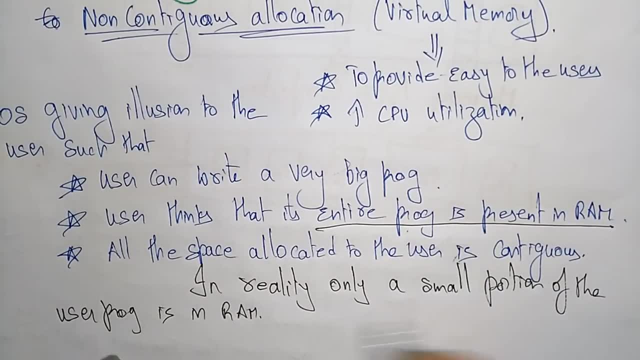 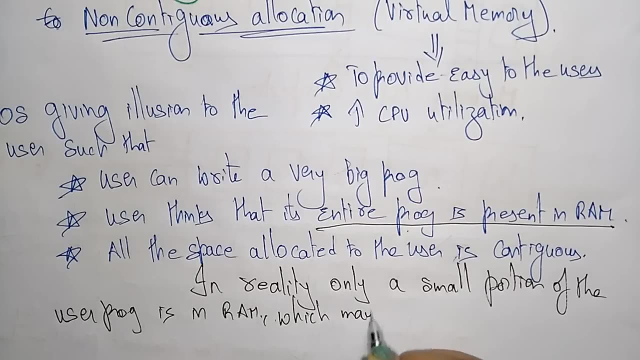 we are. we are having only just the illusion means we are adding some virtual memory, but in reality only the small portion. whatever we want to be executed, that small portion of the user program is in ram with the help of the library functions, so which may or may not be contiguous, so that 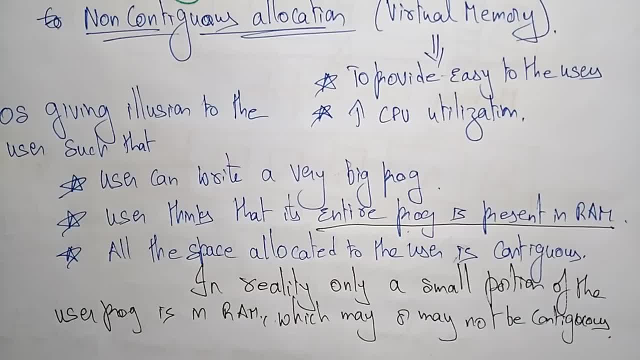 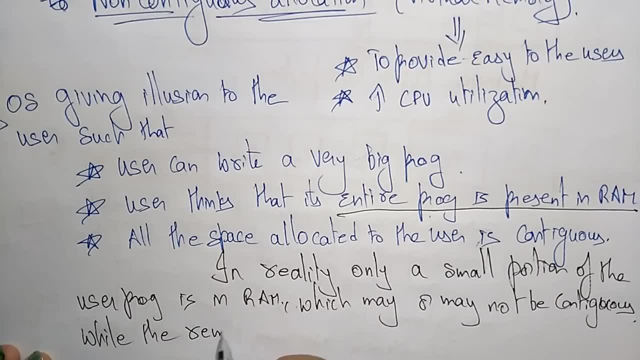 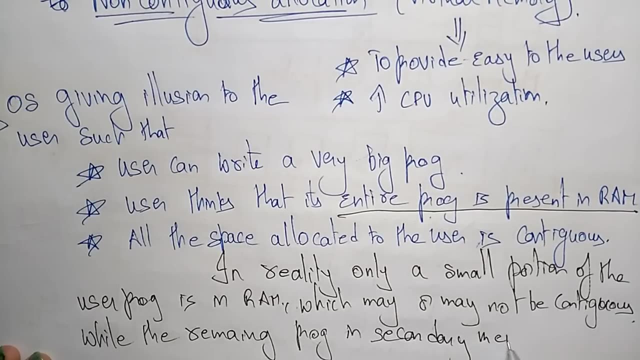 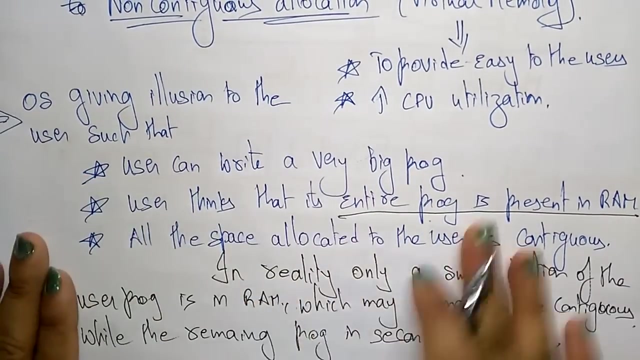 whatever the data, that small portion that you are using that may or may not be contiguous, while the remaining program is present in secondary memory, while the remaining program in secondary memory. so if you know this concept, then you can understand the paging concept. actually here what i am saying, that a non-contiguous allocation is also called. 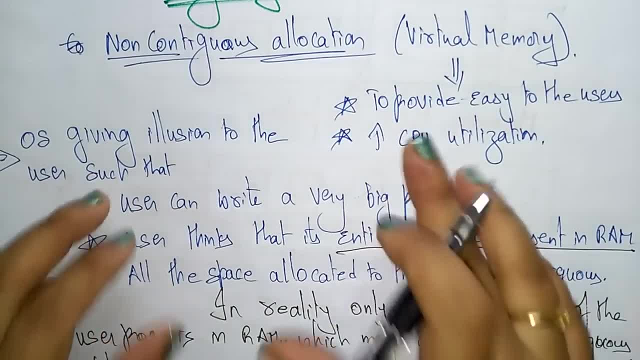 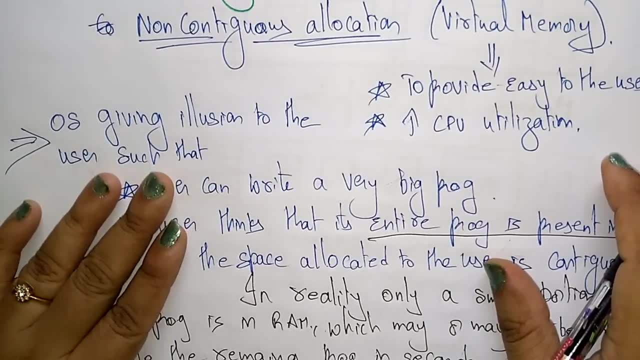 as a virtual memory. actually, this virtual memory why we are using to provide ease to the users and to increase the cpu utilization. how it is increasing the cpu utilization, it's just giving an illusion to the users such that user can user thought that we are writing a very 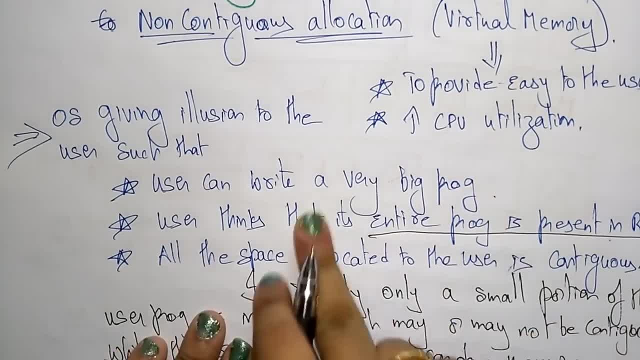 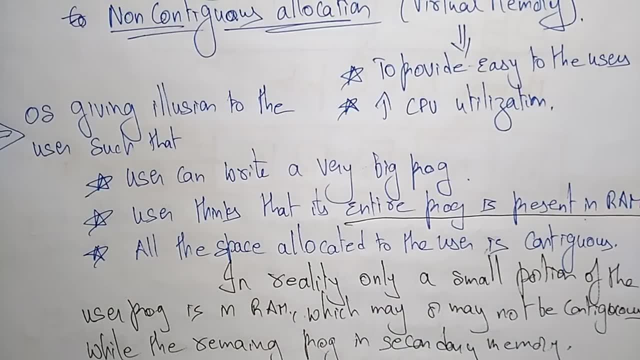 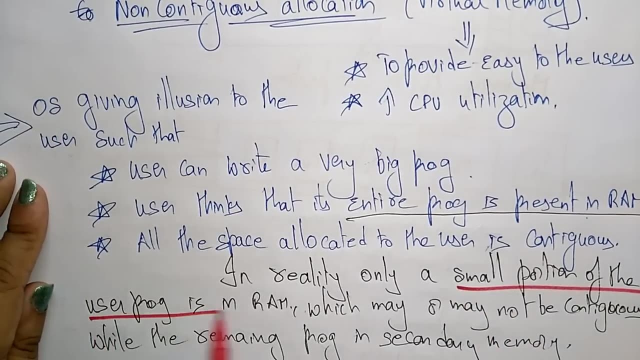 big program so that complete, the that complete, uh, big program is to store in the ram and there is a space that is allocated to the user is contiguous. so we are just giving its illusion, but in reality only a small portion of the user program is stored, only the small portion of user. 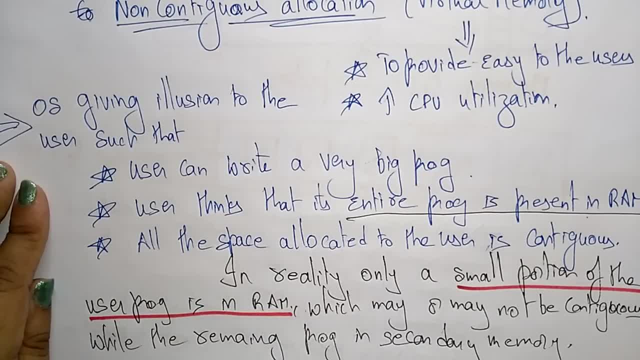 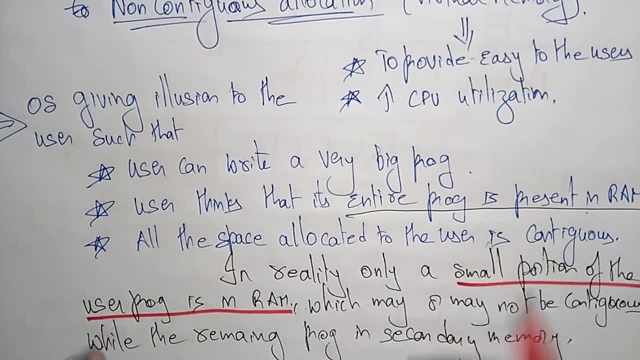 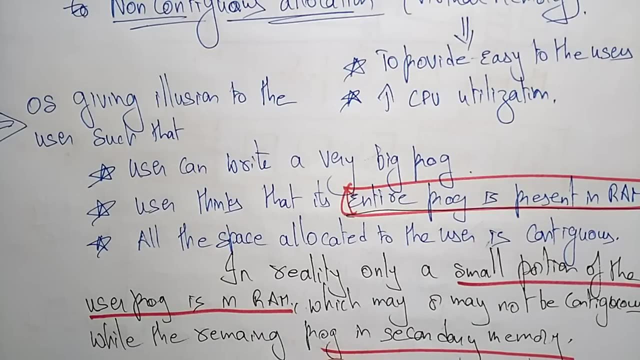 program is present in ram and that may be contiguous or non-contiguous, whatever it may be, but only the small portion of user program is in ram and the remaining program the entire. in this entire program, only small portion is stored in ram and the remaining program is stored in secondary memory. 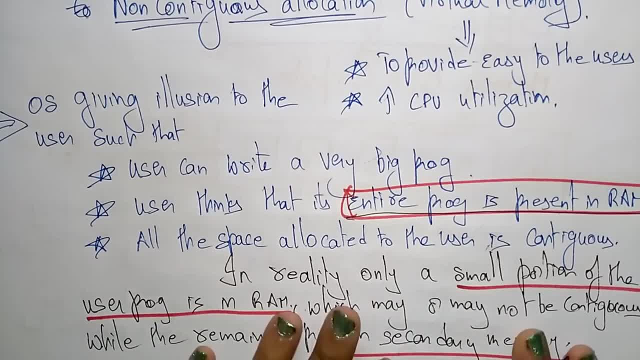 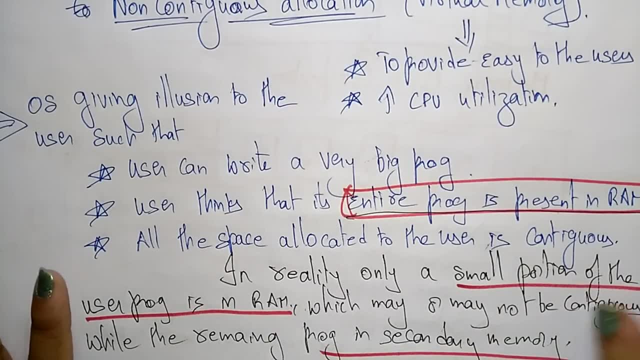 so actually that is a concept. only small program stored in remaining program is stored in secondary memory, but we thought that the entire program, whatever we are returning that- completely stored in ram. so now coming to the concept paging. so what here the paging means? and i'm talking about this? 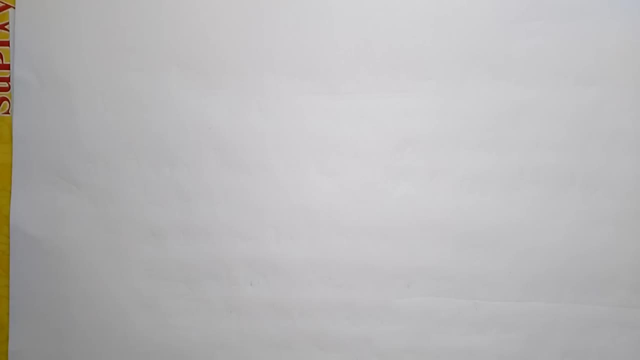 virtual memory. uh, why, it is related to this page. now let me write that. so here the main memory is divided into number of equal size, relatively small frames. so here the process is loaded by loading all its pages into available frames. so let me write that: a computer, 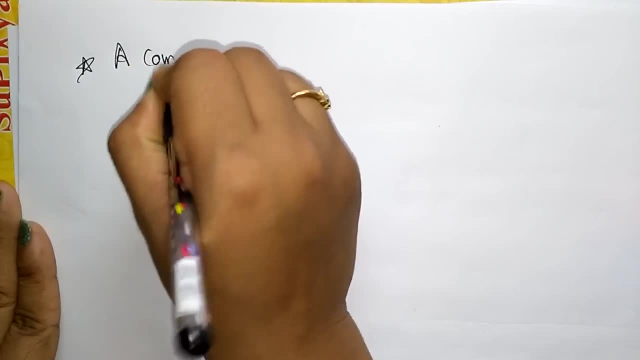 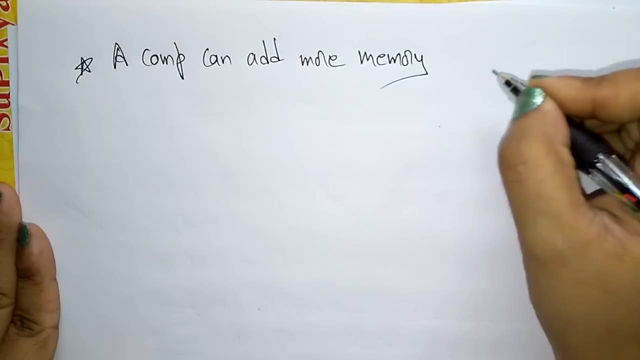 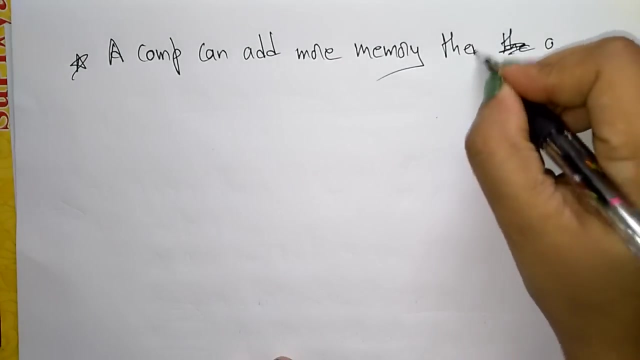 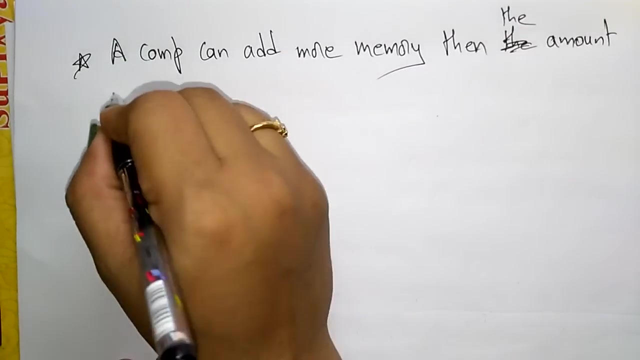 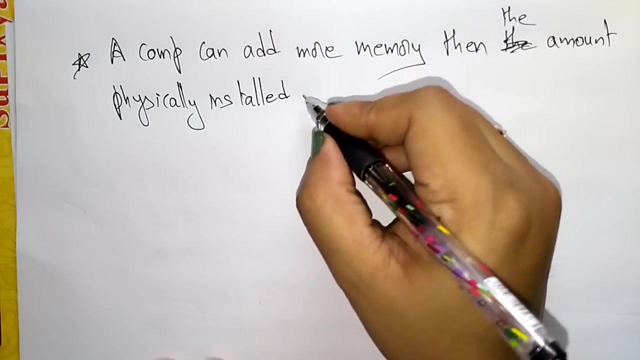 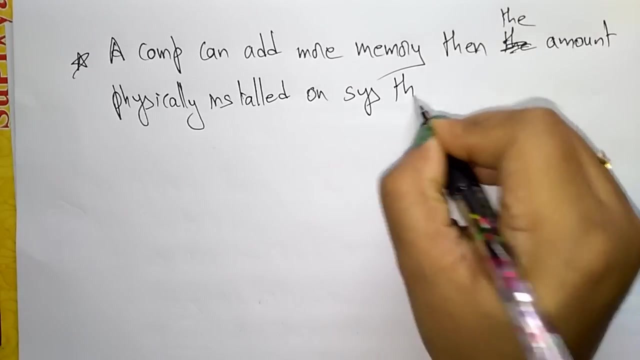 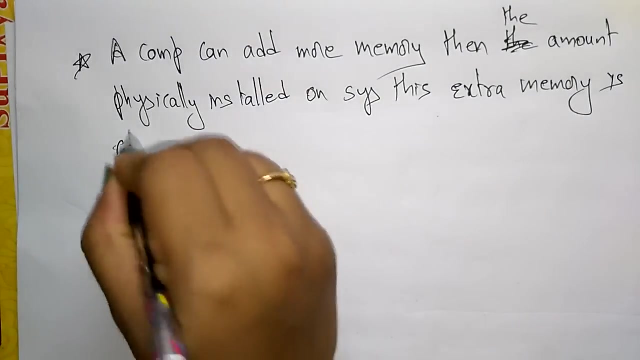 a computer can add more memory. a computer can add more memory than the memory, than the amount of, sorry, than the amount physically installed, physically installed on system, on system. this extra memory is called, this extra memory is called. this extra memory is called, is called virtual memory, is called virtual memory. 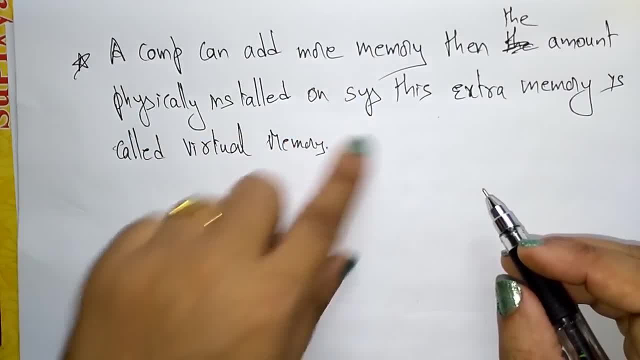 is called virtual memory. so in a computer a computer can add more. so in a computer a computer can add more. so in a computer a computer can add more memory than the amount of physically memory, than the amount of physically memory, than the amount of physically installed. suppose already we thought, 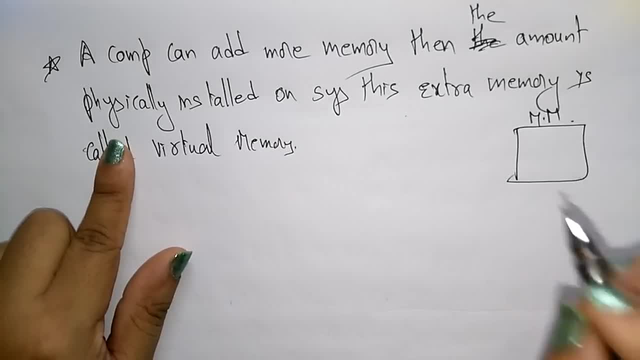 installed, suppose already we thought. installed, suppose already we thought that the main memory is uh the size of that. the main memory is uh the size of that. the main memory is uh the size of the main memory. it can store up to 64. the main memory, it can store up to 64. 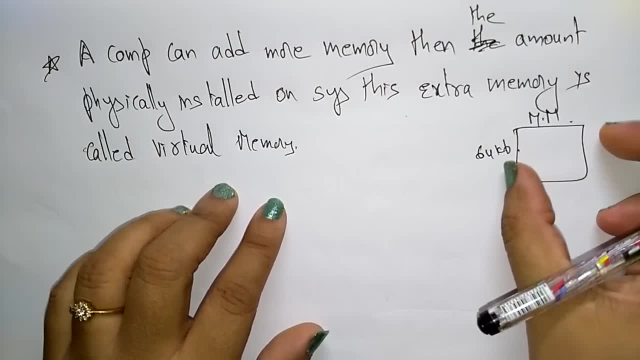 the main memory. it can store up to 64 kilo kilo kilo. 64 kb. so it can stored 64 kb. so it can stored 64 kb. so it can stored 64 kb of size of memory. 64 kb of size of memory. 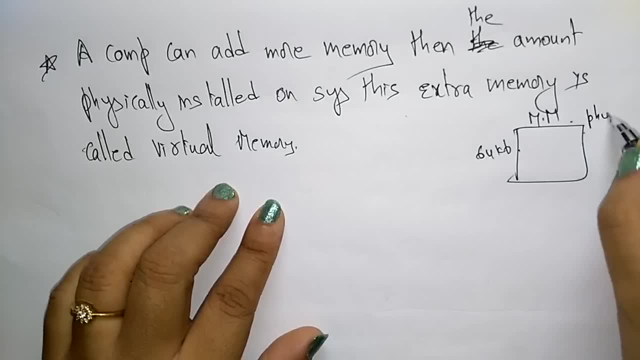 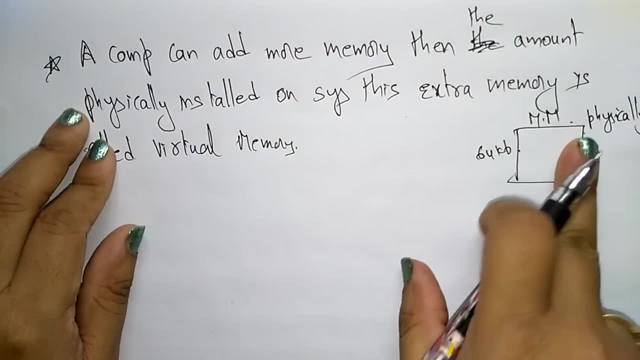 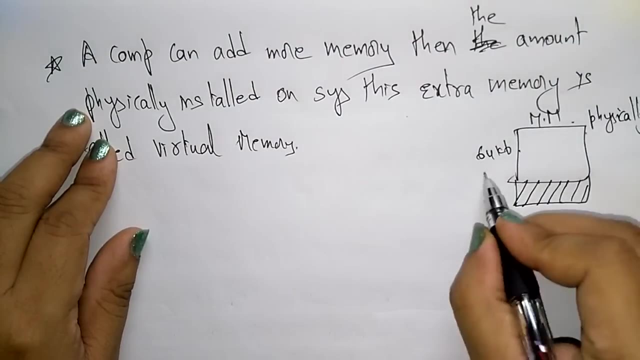 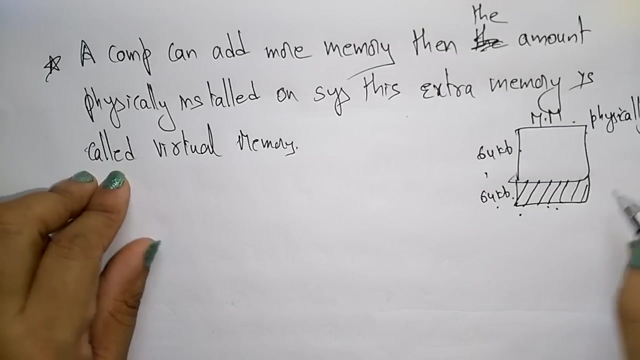 size of memory. so this is physically installed. physically installed, we thought that it is physically installed so a computer can add more memory than the amount of physically memory on system. uh, so it can add more memory already physically installed- 64 kb. so again, i want to add some 64 kb. okay, so this extra memory, you call it as a virtual memory, virtual memory actually. 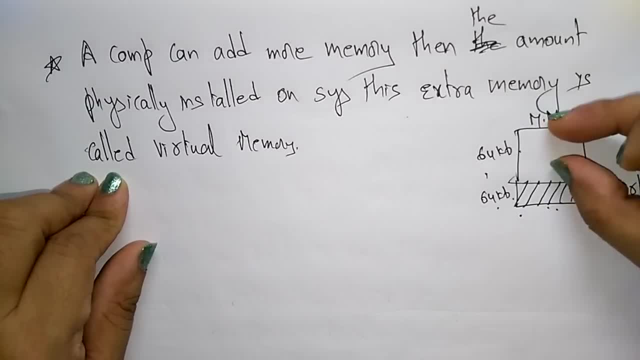 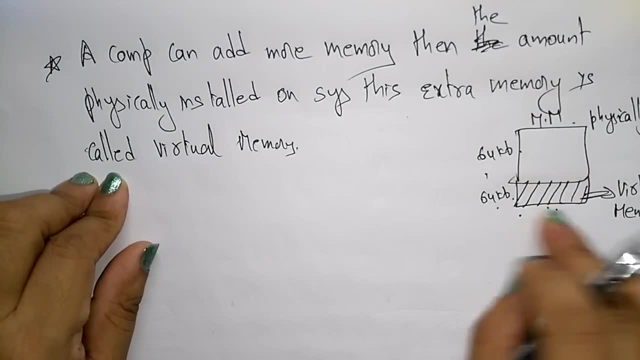 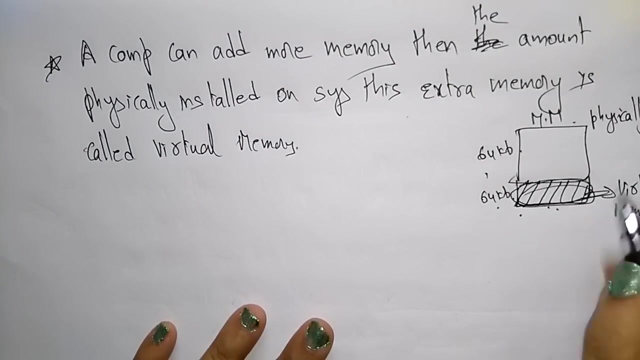 this is not real. okay, so this, only the 64 kb. whatever it is, the physically installed main memory is 64 kb and this is an illusion. here we want to store the temporary uh data, just uh. it's only. whenever the system is off, the whatever the memory that is there, this completely erased and 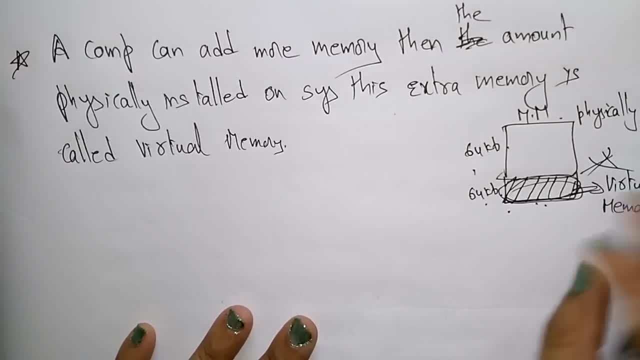 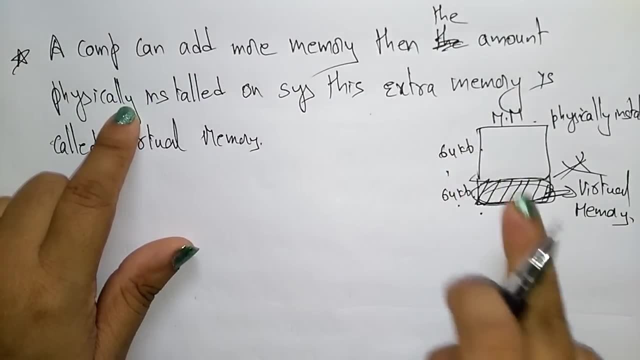 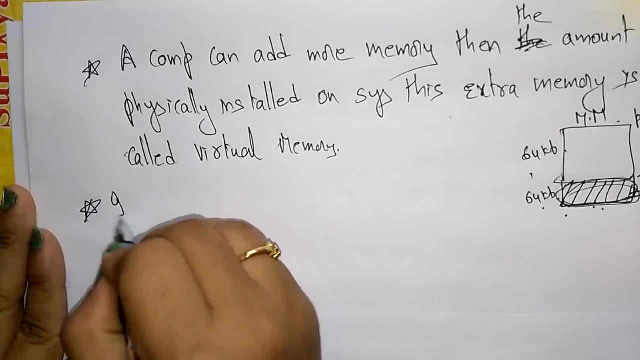 this will be discarded. okay, so this concept, you call it as a virtual memory. a computer can add more memory than the amount of physically installed on the system. this extra memory is called as a virtual memory. it is a memory management technique. so a paging is a memory management technique. 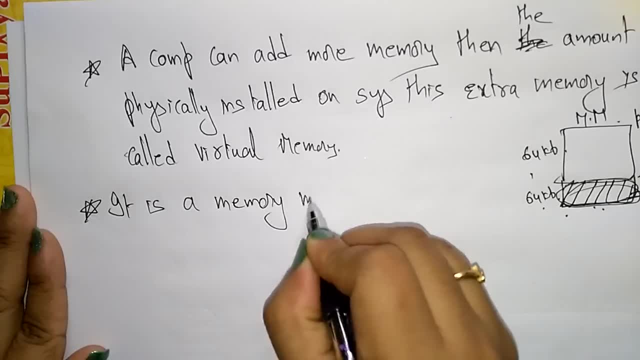 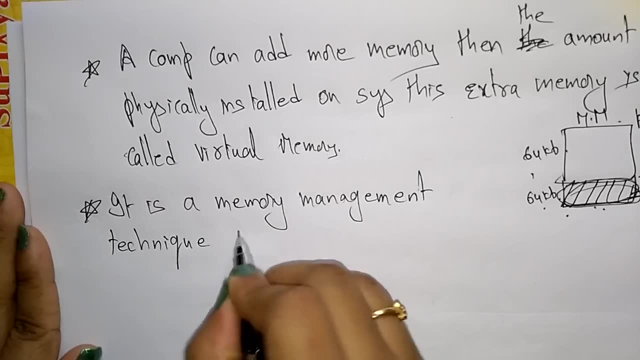 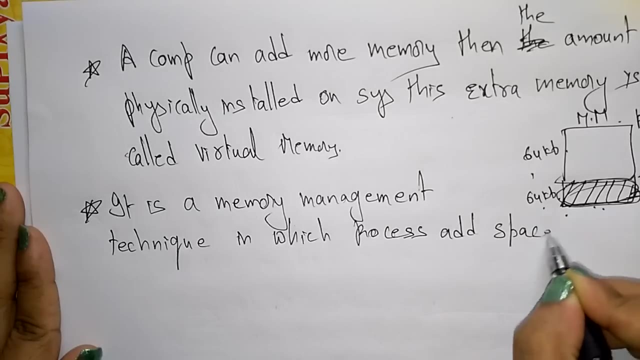 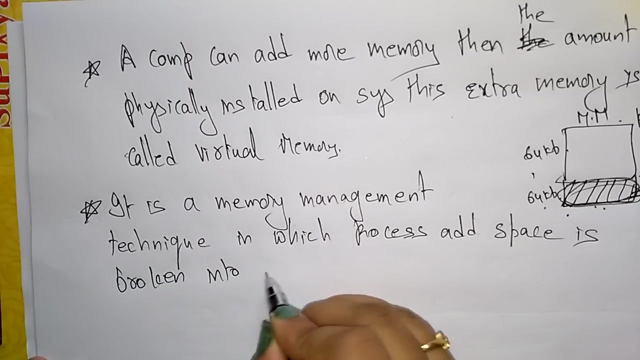 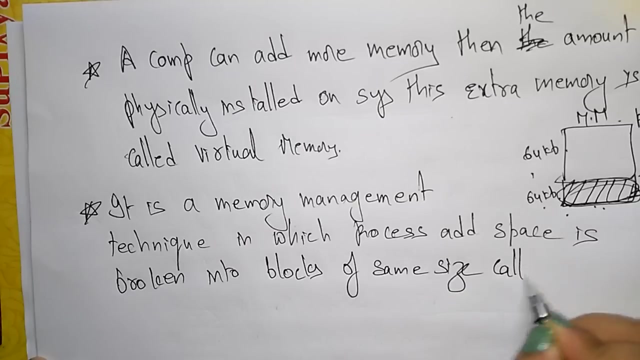 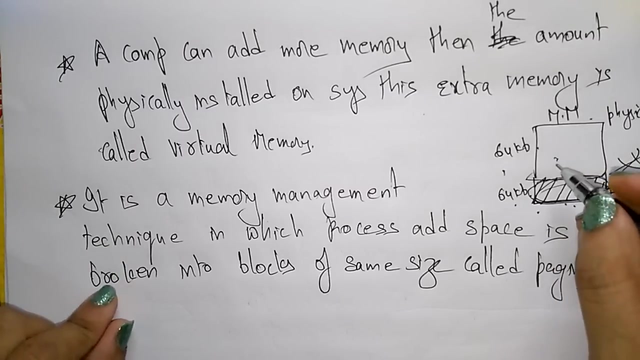 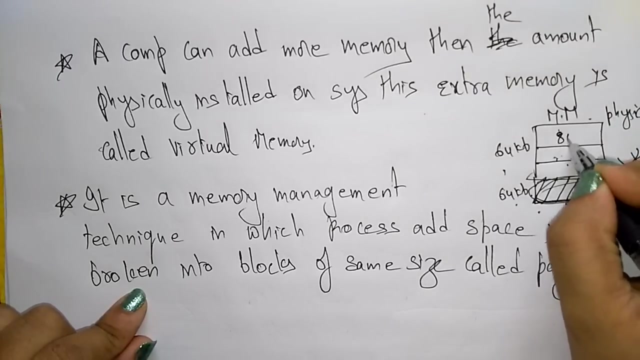 in which process add space is broken into blocks, divided into into blocks of same size, called paging. so this here the memory is there. so this memory in which the process address space is broken into blocks, blocks of same size. so this is suppose 8 m 8. 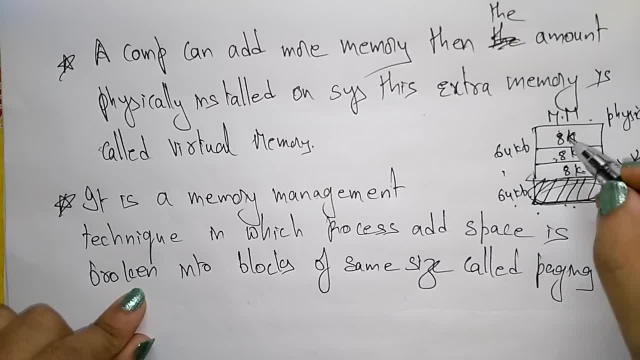 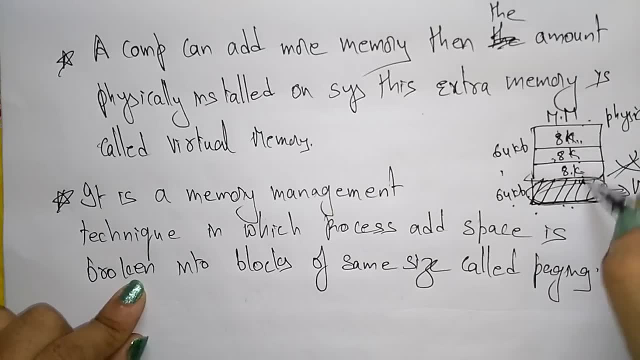 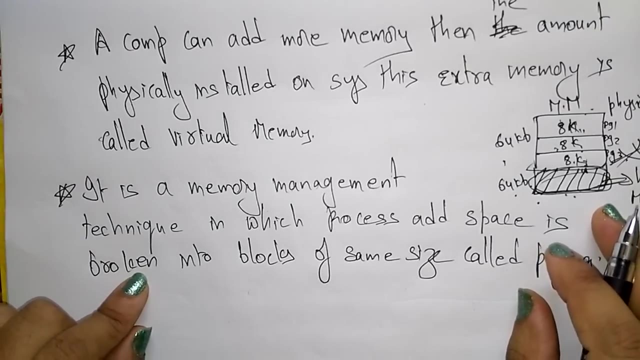 kilobytes, 8 kilobytes, 8 kilobytes, like that. so uh, in which a process, address space is broken into, is broken into blocks of same size, blocks of same size. this is called paging page one, page two, page three, like that. okay, so here the size of the size is just the page size is of power of two. it's. 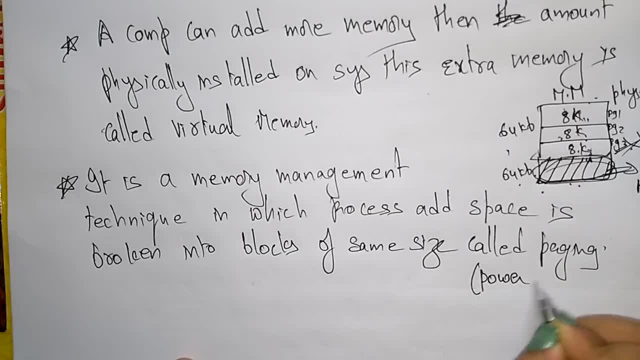 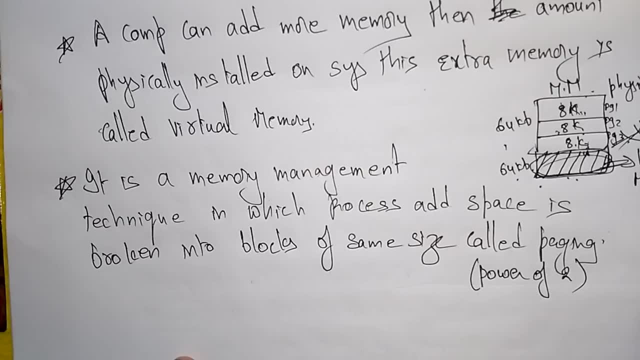 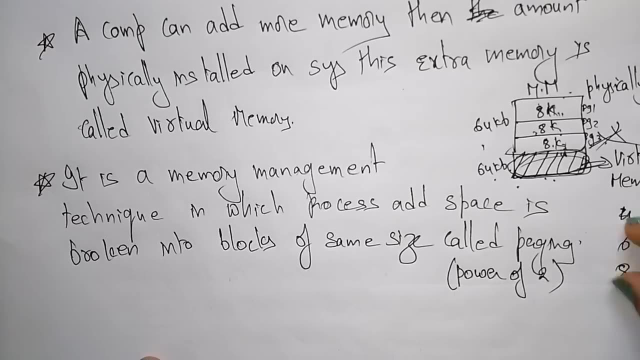 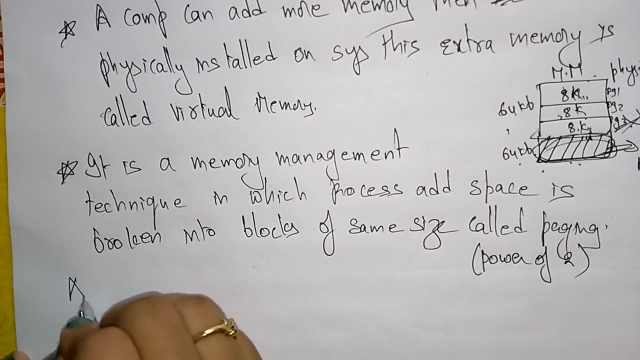 always in the size, should be power of two, either two, four, six, like that, eight, two, four, six, eight, like that. so the paging space, the block size, will be the always the powers of two. so the size of process is measured in with the help of number of pages, always the size of. how can we say that? what? 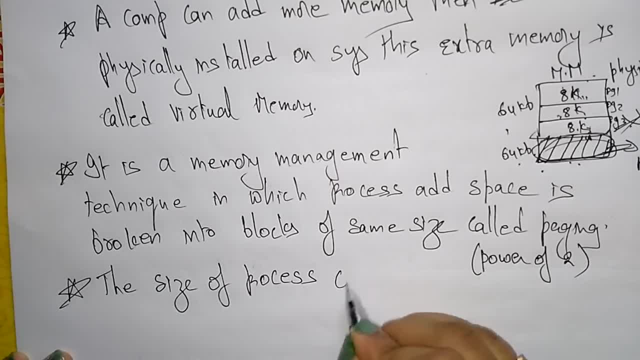 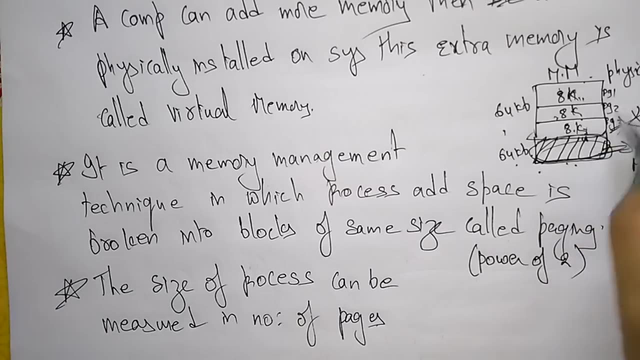 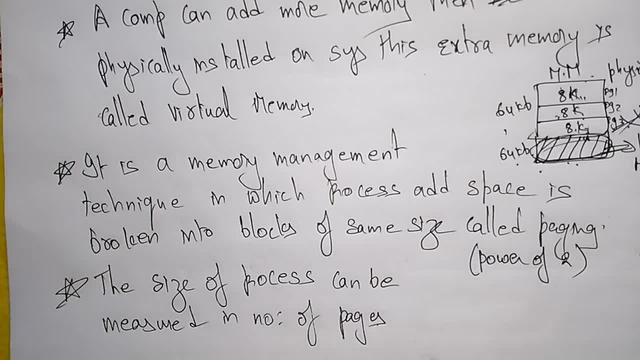 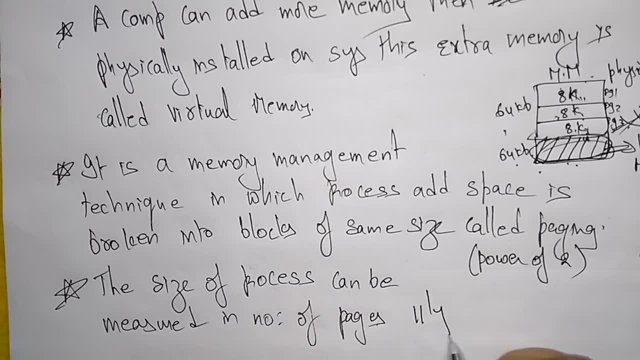 be measured in number of pages. so, similarly, a main memory is divided into small, fixed size of blocks. that is the physique. let me write that. similarly, a main memory is divided into Use of Additional main memory is divided into small size of the block. size of paging page one page, two pages.